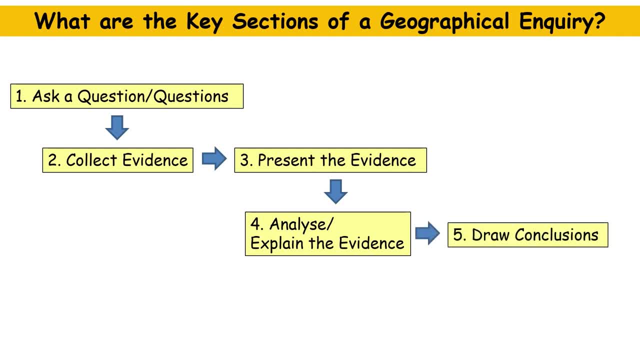 We draw conclusions, which you can do. We draw conclusions which is a summary of what we found out, And then we might do an evaluation section where we say what went well and how we could improve it. Now the fieldwork part of all of this is that stage two. 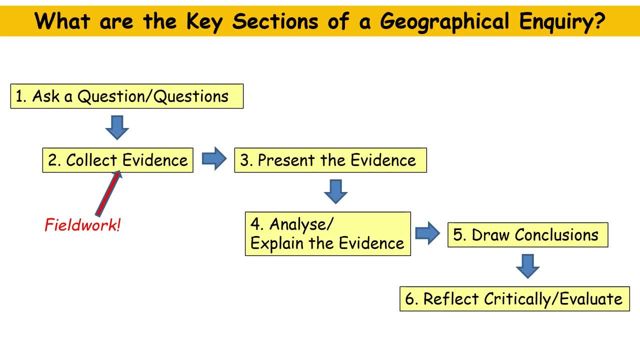 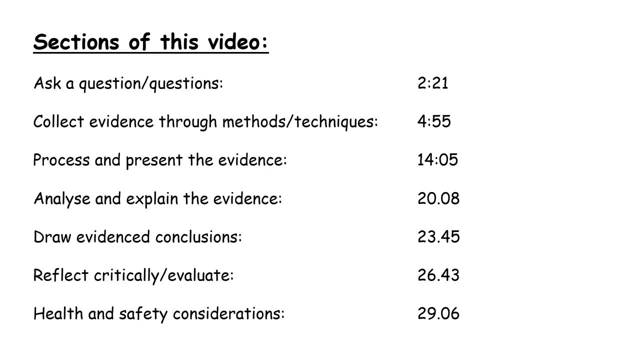 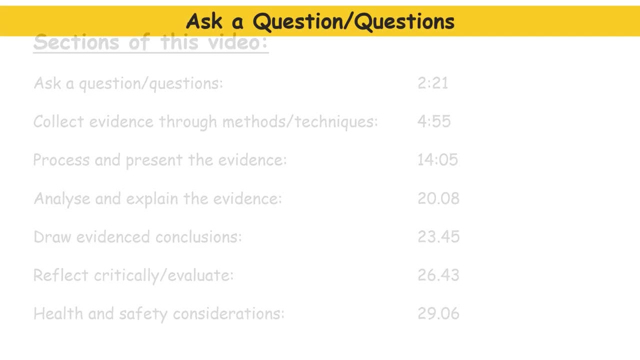 It's the collecting evidence bit. The rest of this video goes through each part of the inquiry process. You can see the timings below, so it's easy to skip to a section that interests you. The first section of our inquiry is about the questions that you might ask. 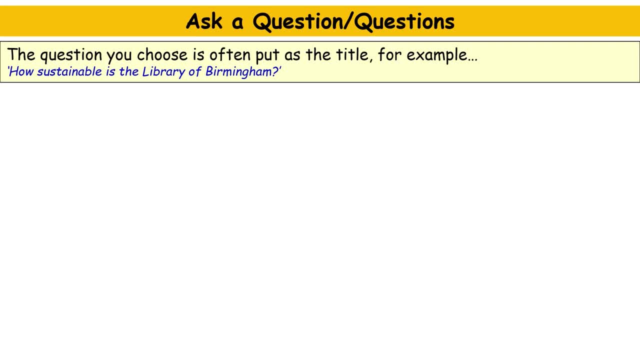 Normally people put the question as the title of their inquiry. So here it is: How sustainable is the Library of Birmingham? It's a question and a title. Often people split the key question into aims. So aim one to investigate whether the Library of Birmingham is socially sustainable. 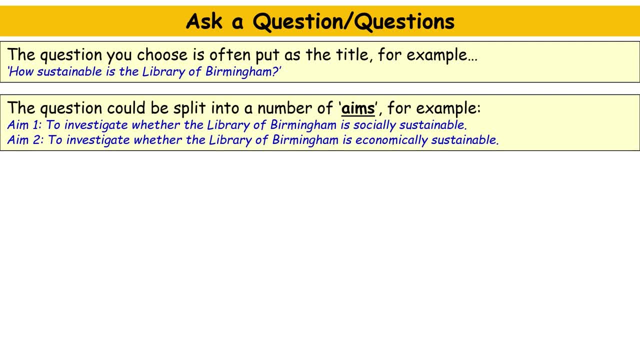 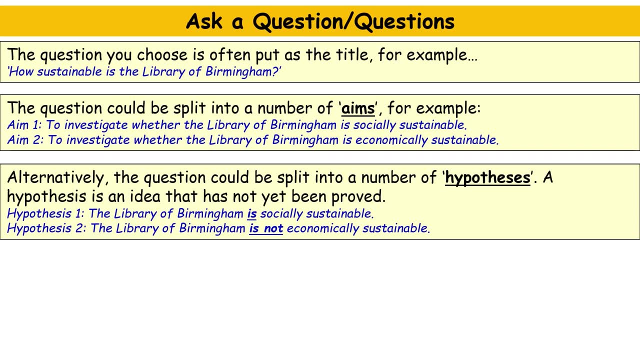 Or aim two, to investigate whether the Library of Birmingham is socially sustainable. Or aim three, to investigate whether the Library of Birmingham is economically sustainable. Alternatively, people split the question into a number of hypotheses, Hypotheses being ideas that have not yet been proved. 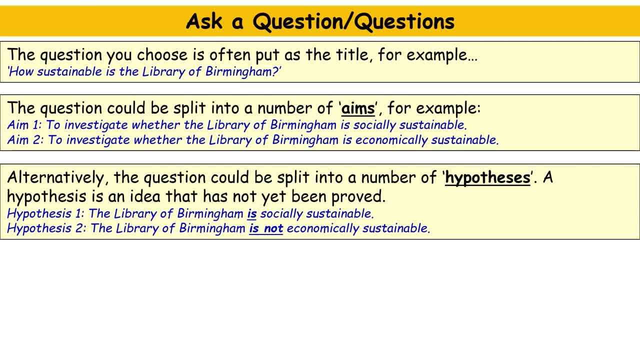 So with our example, hypothesis one: the Library of Birmingham is socially sustainable. You'd go away and during your fieldwork you'd be able to prove whether it is or it isn't. Hypothesis two: the Library of Birmingham is not economically sustainable. 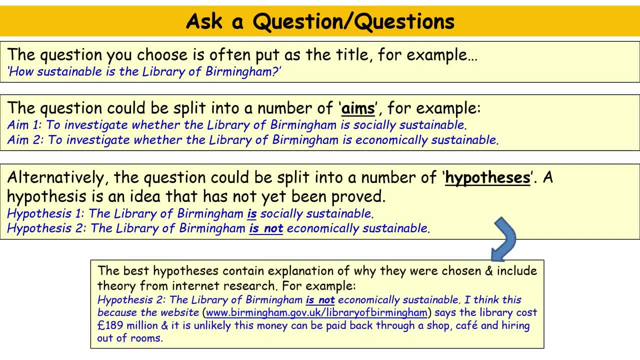 Now, the best hypotheses that you could write contain a bit of explanation of why they were chosen and might include a bit of theory. So the Library of Birmingham is not economically sustainable. I think this because a certain website says the library costs £189 million. 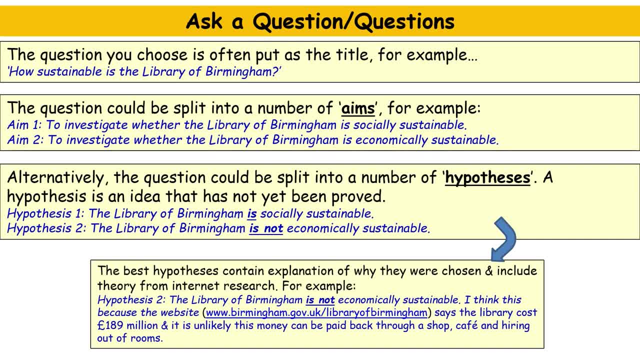 And it's unlikely this money can be paid back through a shop, cafe and hiring out of rooms. So normally, with the hypotheses, you've done some internet research, you've done some background reading, you've come up with something, But then you're going to go and test when you do your fieldwork. 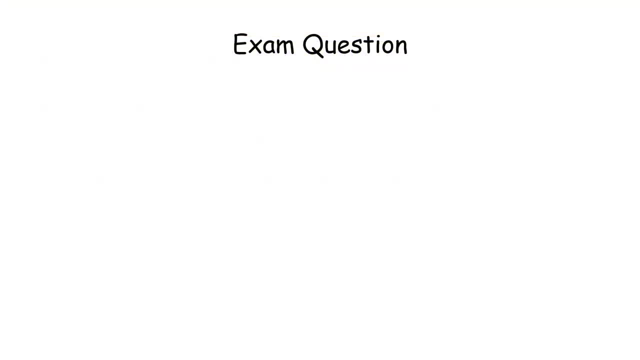 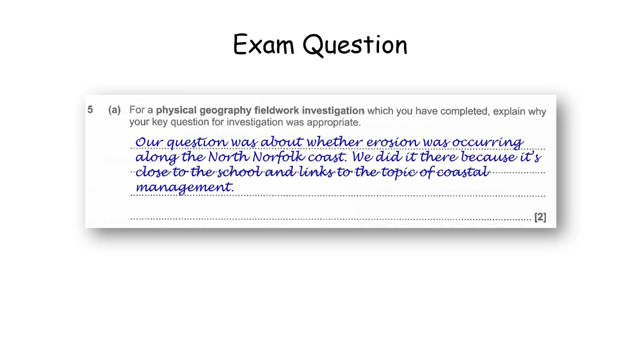 Here's an example exam question. So, for a physical geography fieldwork investigation which you've completed, explain why your key question for investigation was appropriate. Now they have been studying whether erosion is occurring along the North Norfolk coast. They're saying it's appropriate because it's close to their school. 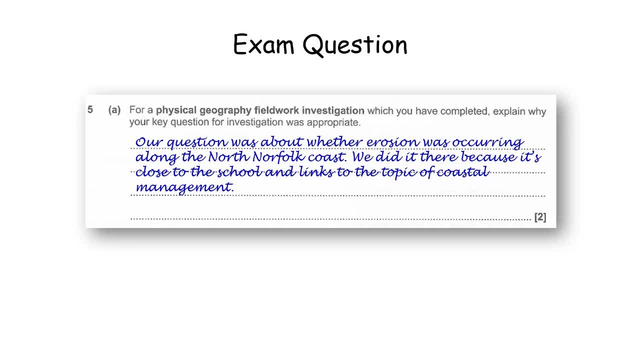 That makes sense. They can do it within one day And it links the topic of coastal management. That makes sense. They've got the theory about this topic because they've learned about it as part of the syllabus. That's why that is worth two marks. 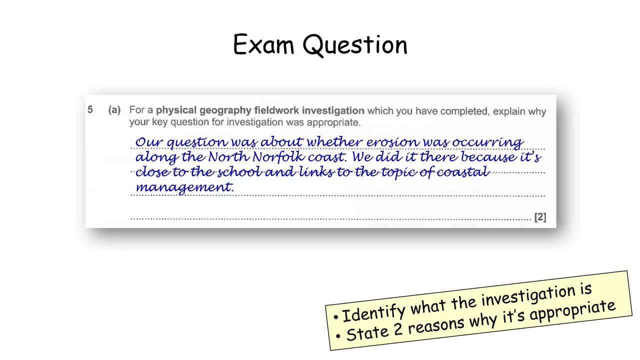 So, in summary, they've identified what the investigation is and they stated two reasons why it's appropriate. Now, if they're not asking about your own fieldwork and they're giving you an example of fieldwork and asking you to write about it, do the same. 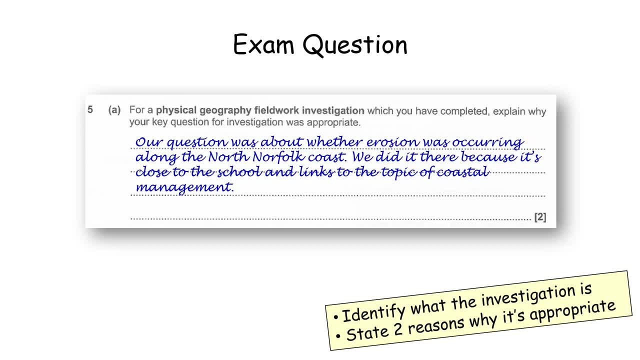 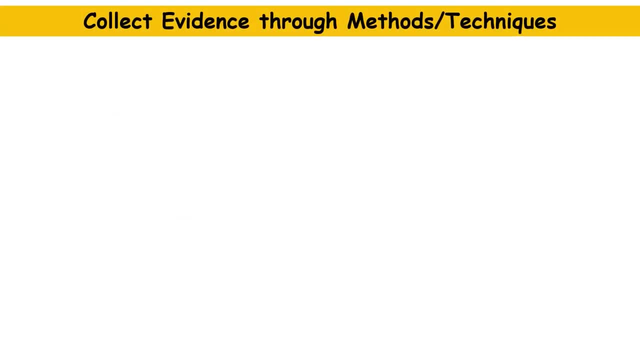 Is the question appropriate? Does it fit in with the fact that they could get there and back in one day? Is it something they've learned about? Can you get good hypotheses and conclusions from what they're learning about That sort of thing? Collecting evidence: the methods section. 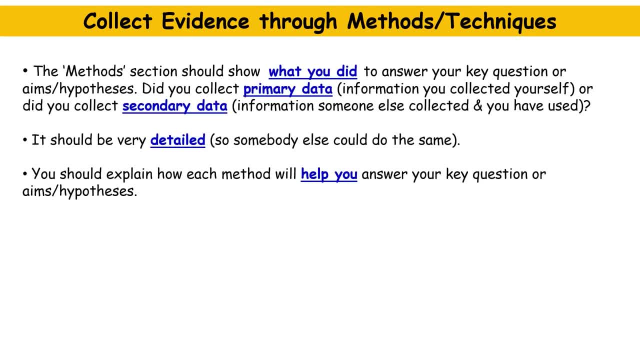 Now in the methods section, you just write what you did to be able to answer your key question. Did you do a traffic count? Did you do a questionnaire? Write whether you collected primary data. That's stuff that you collected yourself, Or did you do. 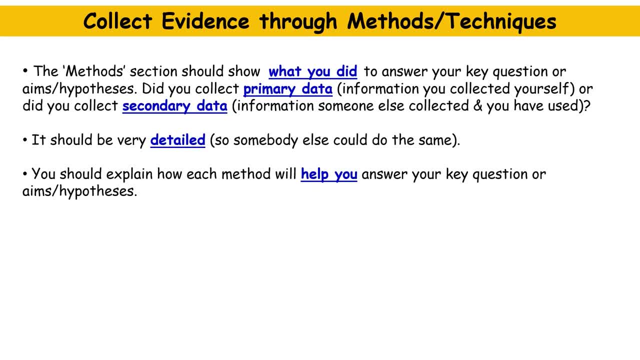 And your investigation with secondary data, And that's where you're using someone else's information. Usually, the secondary data is all of your Internet research. It's great, There's no problems with it. You're using information someone else has provided. It should be very detailed So someone else could do the same method. 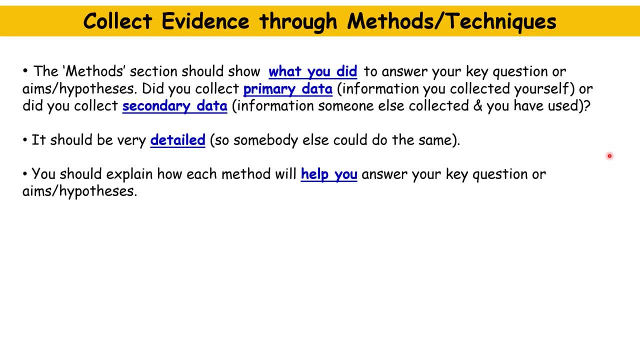 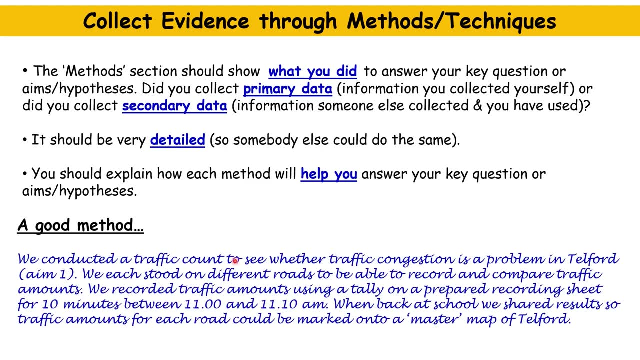 They could copy exactly what you have done and explain how each method will help you answer your key question. That shows the reader, The reader of the project, how it's relevant. Now here is a very good method as an example. They've told us what they did. They did a traffic count. 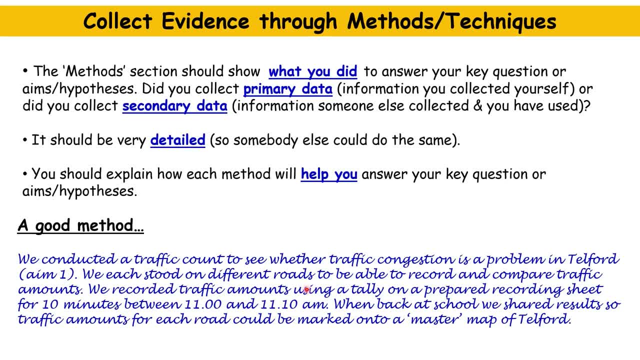 But then they've added the detail. They've said they stood on different roads. They've said they recorded it using a tally. They've said they had a prepared recording sheet. They've also linked it into their aim. They've said they're doing it so they can see whether traffic congestion is a problem. 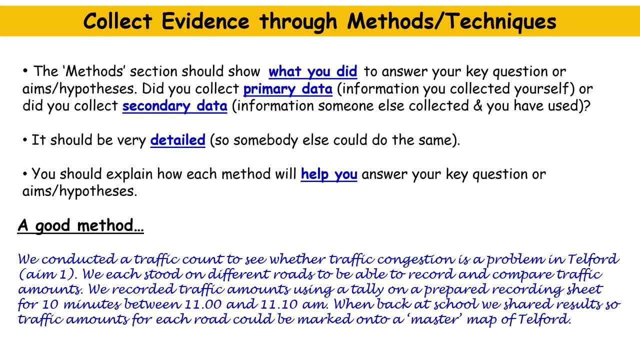 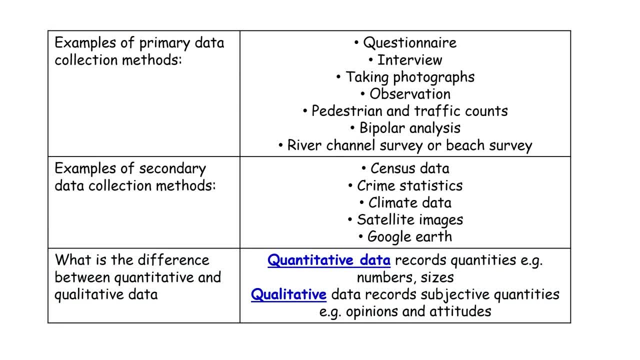 Is a problem in Telford. Now, what they've done, the detail explaining why they've done it, That makes a good method. Here are some examples of different methods that might be used. These are primary data methods, So these are ones where you go out to get your own information. 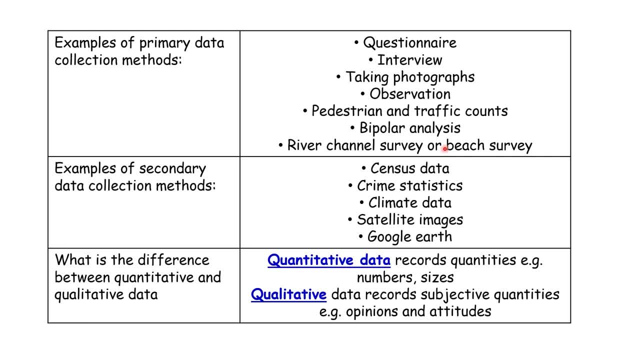 You might visit a river and do a survey. You might go into a pedestrian count or a traffic count. You might observe or take photos Or do interviews or questionnaires. Secondary data: You might use information you can get from the Internet or elsewhere. 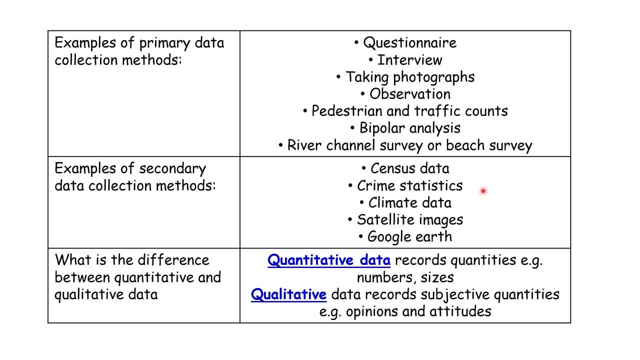 such as census data or crime statistics, or satellite images or Google Earth. You might record using quantitative data, That's, precise numbers and amounts, or qualitative data. That's where you're recording your opinions or your attitude. Do you feel there's a lot of crime in an area? 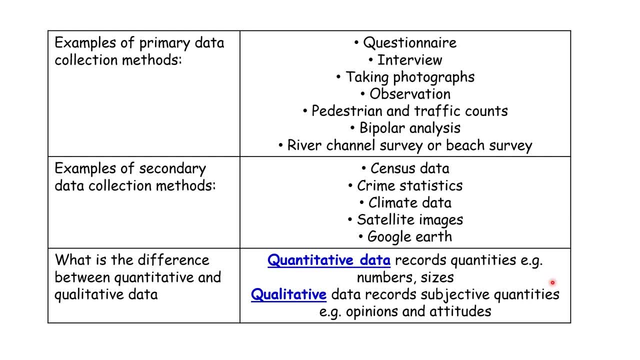 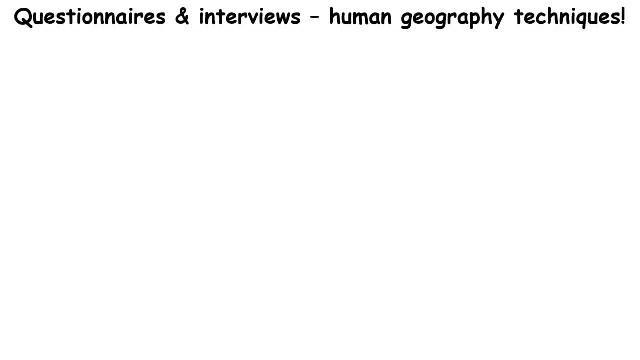 Do you feel it's polluted or congested? So numbers, not involved feelings. Here we're going to look at one human geography method to collect information and one physical geography method. Now we're looking at questionnaires and interviews for our human geography method. 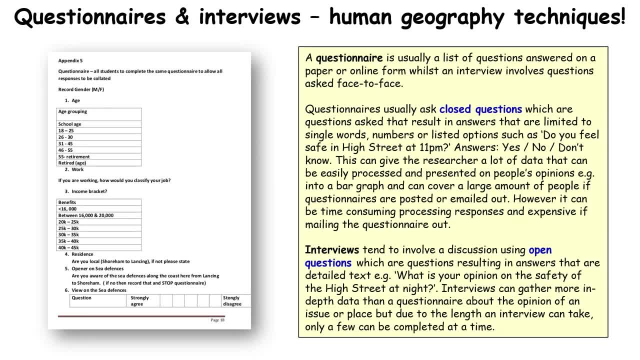 I've gone into it in quite a lot of detail here, in case you're asked about it. So a questionnaire is a list of questions. It's a list of questions answered on paper or online form, whilst an interview involves questions asked face to face. 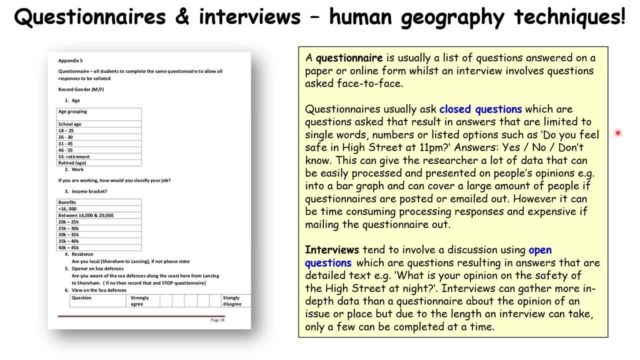 Questionnaires are usually asked closed questions, which are questions asked that result in answers that are limited to single words, And this is done for speed. So it could be something like: do you feel safe in a high street at 11 pm? 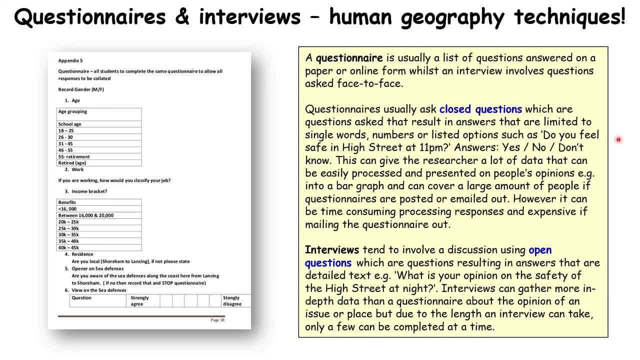 And the person who's being asked rings yes, no or don't know. It gives the researcher a lot of data quickly that can easily be processed. We can easily turn it into graphs And the only problems are it can be quite time consuming. 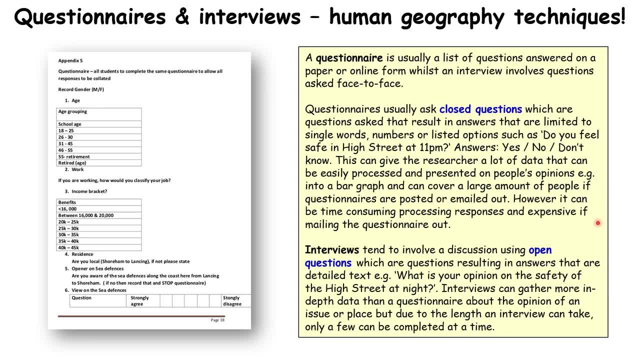 It can be expensive And sometimes you can get quite a small sample size if people don't want to answer them. Interviews involve a discussion with one person where you ask them open questions, So it can be something like: what's your opinion on the safety of the high street at night? 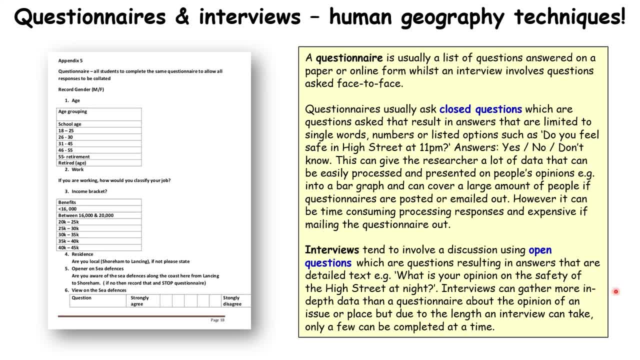 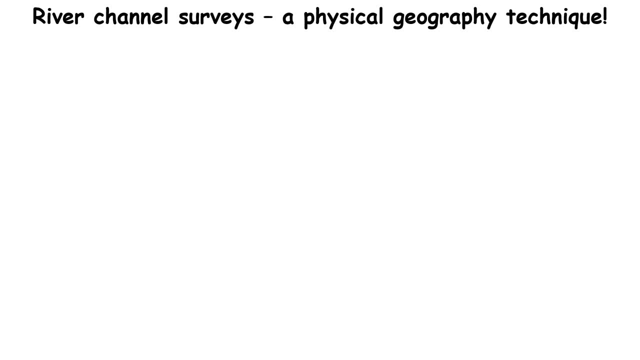 So they can give any response they want. They gather more in-depth information, But due to the length an interview can take, only a few can be completed at a time. Now we'll look at a physical geography technique, which is river channel surveys. 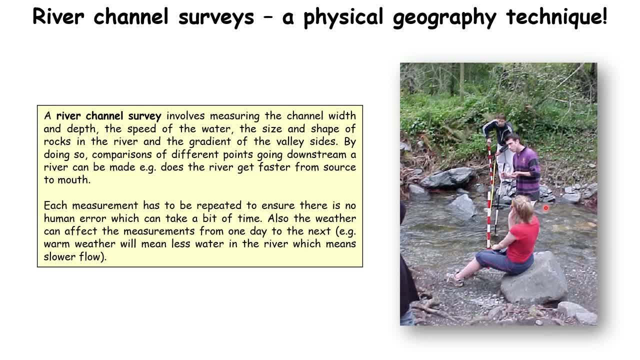 With a river channel survey, you're measuring what the river channel is like at certain places. going down the river's course, You might measure the width or depth or speed of water or the gradient of the valley sides, And if you do this, you can see how the river changes as it goes downstream. 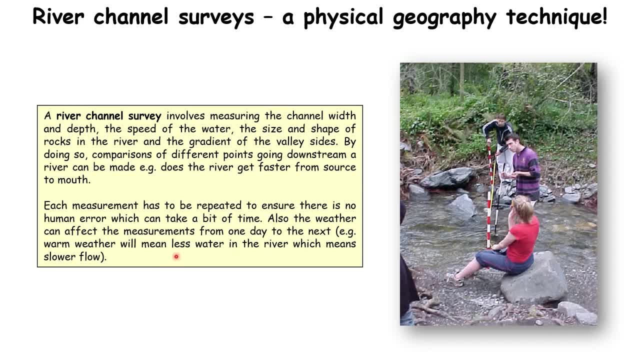 Human error can be a problem with this, especially if you can't trust other members of your group to do things accurately. The weather can be a problem, So here are some examples. Warm weather will mean there's less water in the river, and that would mean a slower flow. 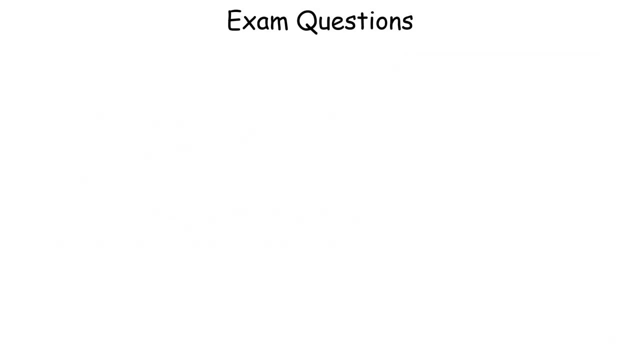 Here are a few past exam questions to do with the methods section. Here's the first one: Justify one technique you used to collect your data And for a human geography fieldwork investigation. justify means: say why you used the technique. So here's an example Questionnaires: is the technique? 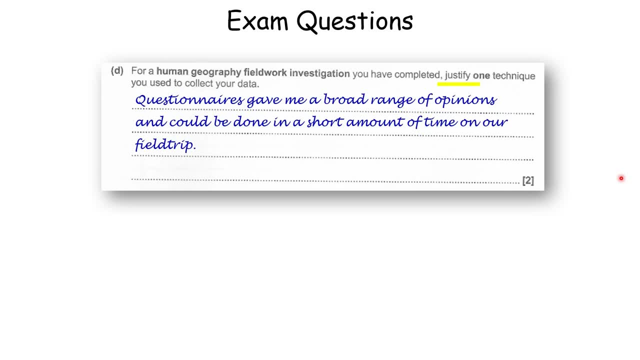 Why? Because it gave me a broad range of opinions and could be done in a short amount of time on our field trip. Perfect. Next Name: a primary data collection technique suitable for carrying out a human geography fieldwork investigation. Looking at the issue of shop closures within an economic hub. 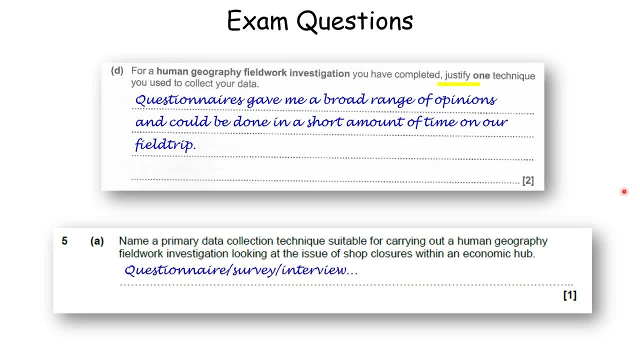 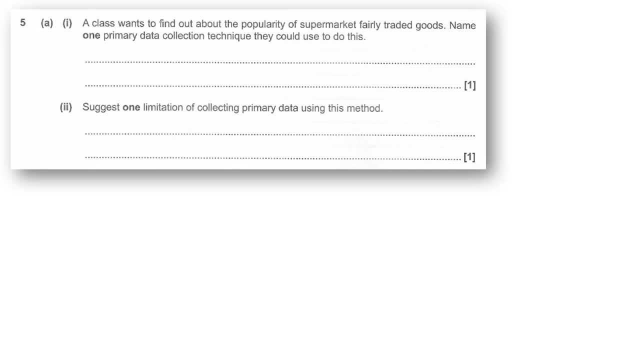 You could say questionnaire, You could say survey, You could say interview. Next, A class wants to find out about the popularity of supermarket fairly trade goods. Name one primary data collection technique they could use to do this Again: questionnaire, survey or interview. 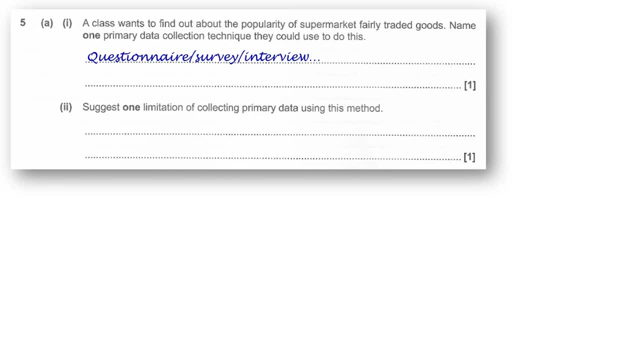 Put one of them, Suggest one limitation of collecting primary data using this method. Well, close questions can provide narrow responses. Or you could say a small sample size may not be representative, Or you might say something like you'd have to visit on different days at different times to make it accurate, etc. 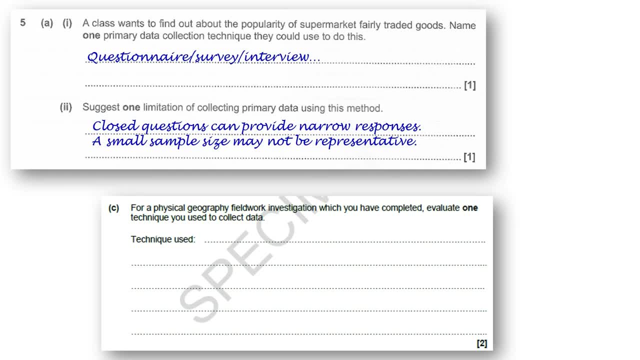 For a physical geography fieldwork investigation, which you have completed. Evaluate one technique you used to collect data. Evaluate means what is the value of it, So what's good and what's bad about the technique that you used? So here's an example. 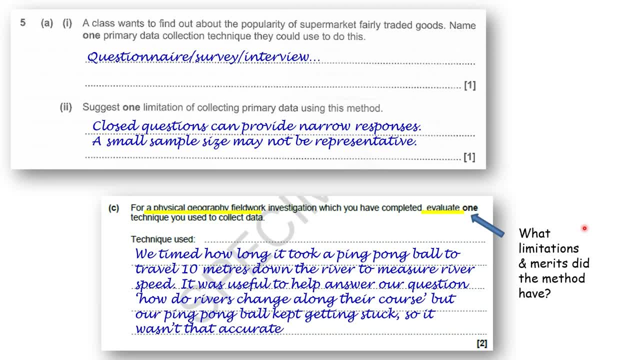 We timed how long it took a ping pong ball to travel 10 meters down the river to measure river speed. And that's great, because you've totally put the examiner in the picture of what your physical geography fieldwork investigation was. Now the good and bad bit. 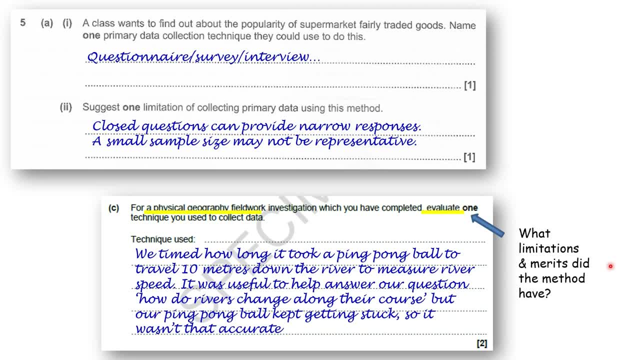 It was useful to help answer our question. How do rivers change along their course? But our ping pong ball kept getting stuck, So it wasn't that accurate. Perfect. Now, if in the exam question they're not asking about your fieldwork, They're giving you an example of fieldwork. 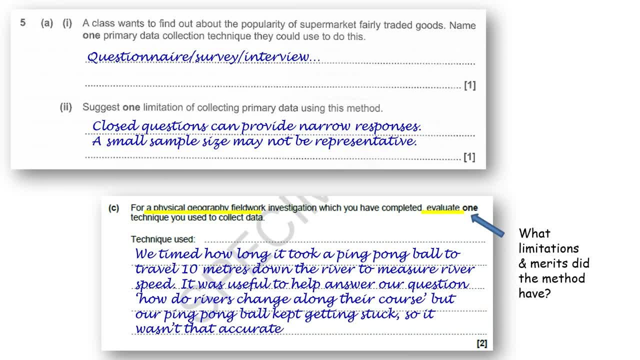 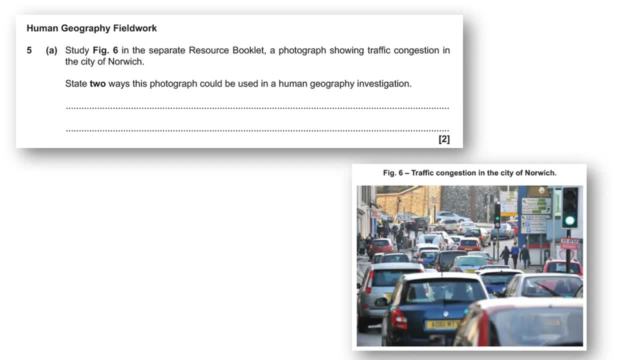 Instead, you could use similar things as answers. Here's a human geography fieldwork example. So here is the photo. This is our resource And we must use the photo if it says: study figure six State two ways. This photograph could be used in a human geography investigation. 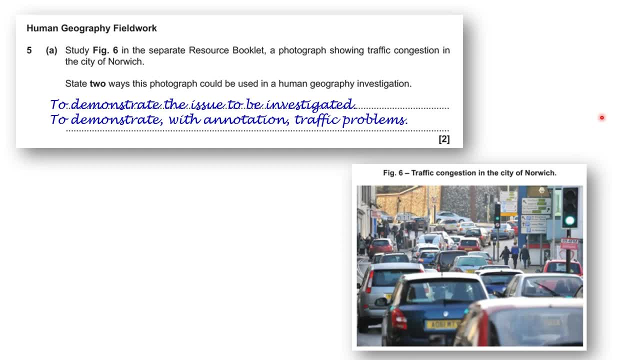 How about to demonstrate the issue to be investigated? One mark. How about to demonstrate, with annotation, traffic problems? Again one mark. Now it has to be something that can be seen within the photo. You can't put air pollution because you can't see it. 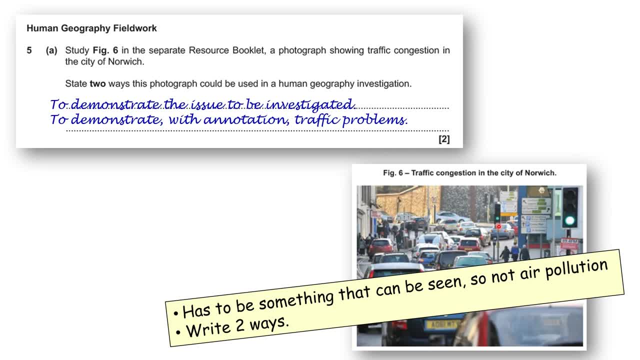 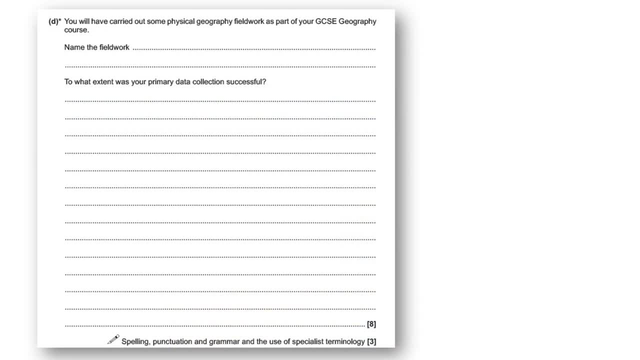 Yes, it might slightly indicate it, but you can't see it. So, with photos, just say things that can be seen. Here's a larger question. You will have carried out some physical geography fieldwork. Or it might say: look at this example of physical geography fieldwork. 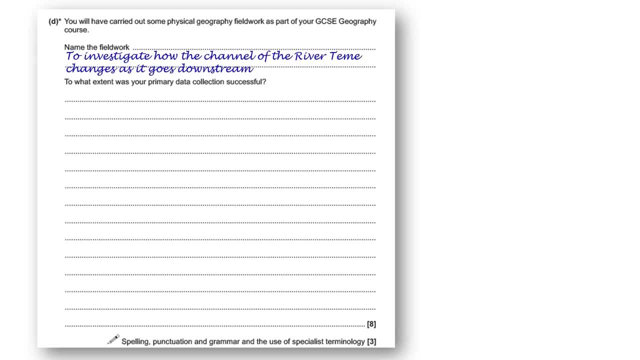 Name the fieldwork. Well, how about to investigate how the channel of the river team changes as it goes downstream? You're telling the examiner exactly what was done. And then, to what extent was your primary data collection successful? Now, with this question, you need to say what went well, what didn't go so well and what didn't go so well. 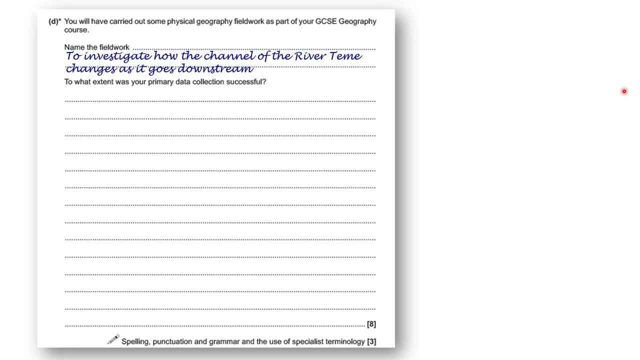 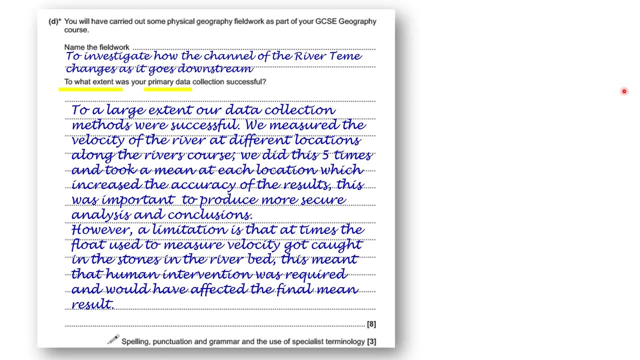 And how it could be improved for next time. So here is a good, developed answer. To a large extent, our data collection methods were successful. We measured the velocity of the river at different locations along the river's course. We did this five times to convene at each location, which increased the accuracy of the results. 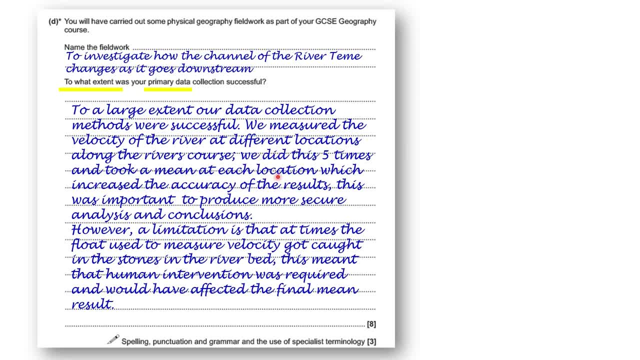 This was important to produce more secure analysis and conclusions. This is great. It's saying what went well And it's also saying how the data that you collected is impacting on your results and conclusions. Next bit, However, a limitation is that at times, the float used to measure velocity got caught in the stones in the riverbed. 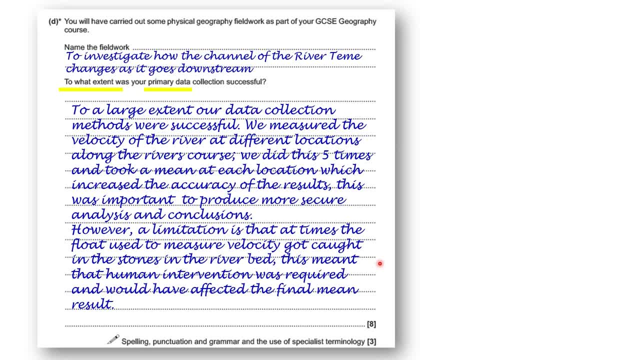 This meant that human intervention was required and would have affected the final mean result. This is great. again, This is saying what didn't go so well. So, to summarise, write what went well. write what didn't go well. Develop your idea. 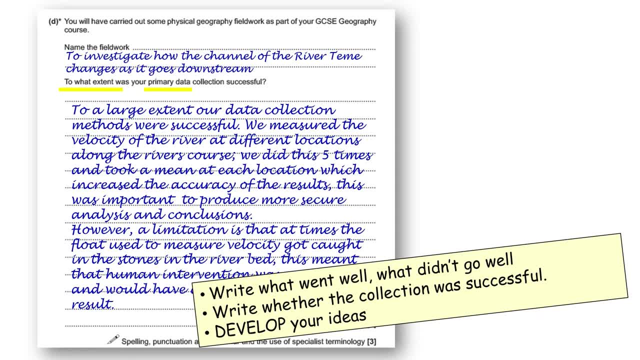 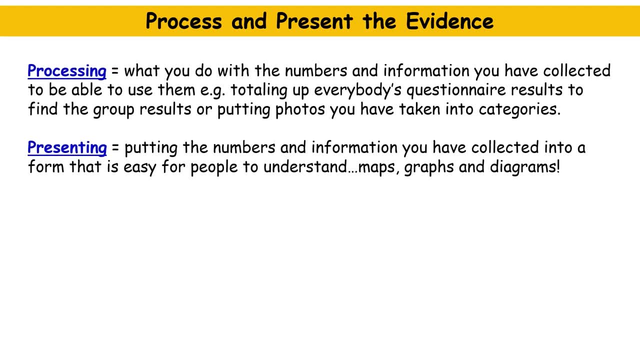 Your ideas And overall write whether the collection was successful or not. Processing and presenting the evidence. Processing is what you do with your numbers and information you've collected to be able to use them. So it might just be toking up everyone's questionnaire results to find the group results. 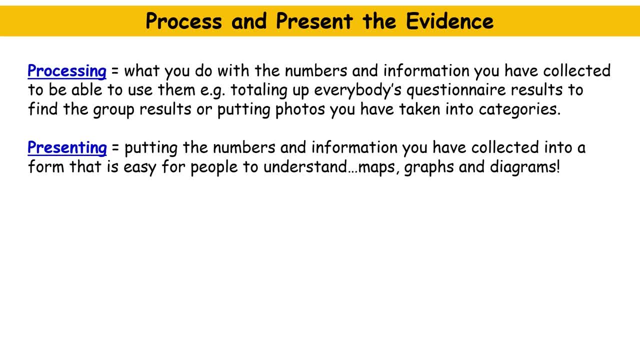 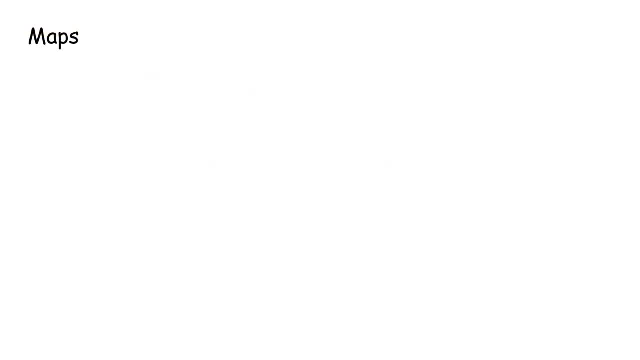 Or you might just take all the photos you've taken and put them into categories to make it easier for you to use them. Presenting the information means turning numbers into maps, Graphs, diagrams, to make it easy for people to understand. I want to focus on each in turn, just to show you what is good. 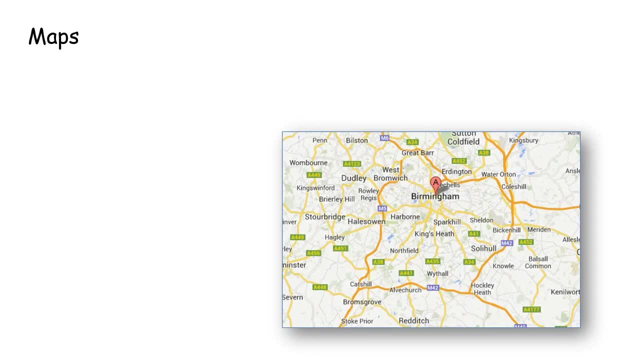 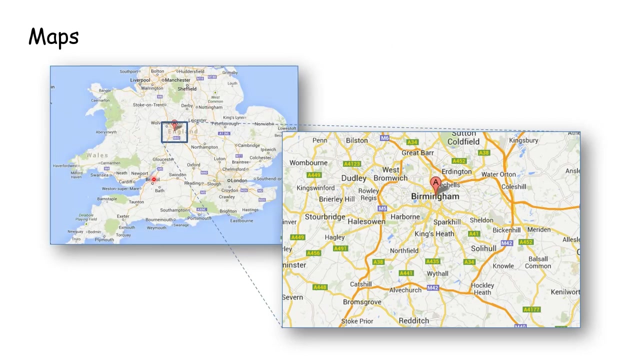 So if you're locating your study area, don't just shove in a map like that. It is useless because to many people who don't live in that area they won't be able to picture where it is in the country. Far, far better if you put in a map of the country. 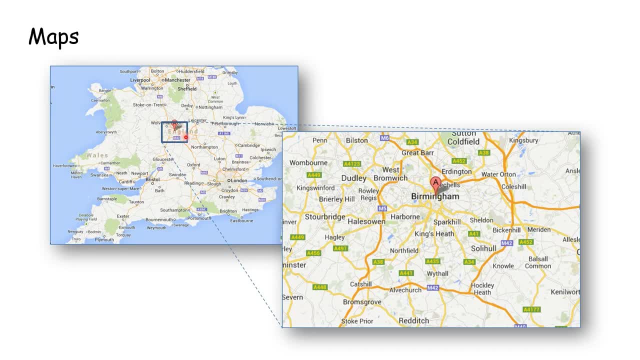 So people think: oh yes, it's that part of the country. Then zoom in on the part that you're interested in. And the same occurs for writing about where something is. Start with locating within the country, Then zoom in and describe where it is in its region. 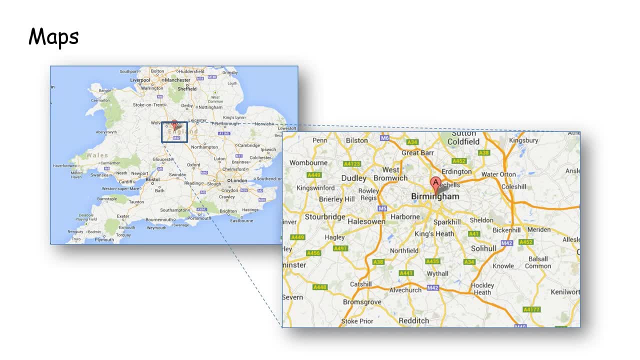 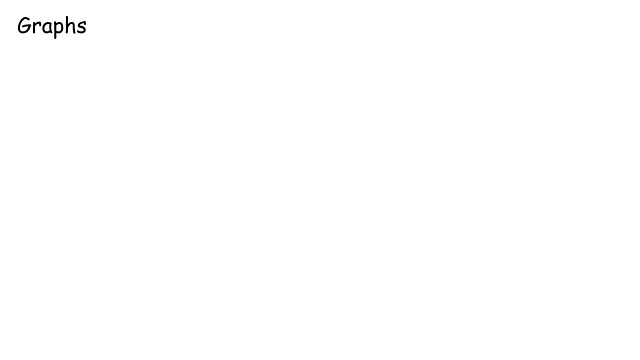 And then, finally, you can go into talking about where it is precisely within a local area. If we're talking about graphs, there are hundreds of different types of graphs That you can do, But for the sake of the GCSE exam, I would just stick with bar chart, line chart, pie chart, the main types. 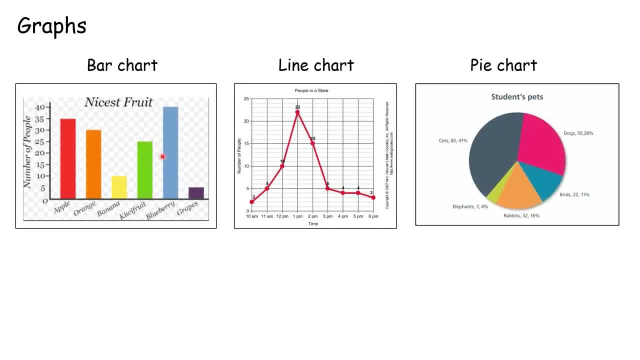 So here is a bar chart showing nicest fruits, Here's a line chart showing changing people in a store over time And here's a pie chart showing people's favourite pets. Bar charts we use to compare things between different groups, So these are groups of people. 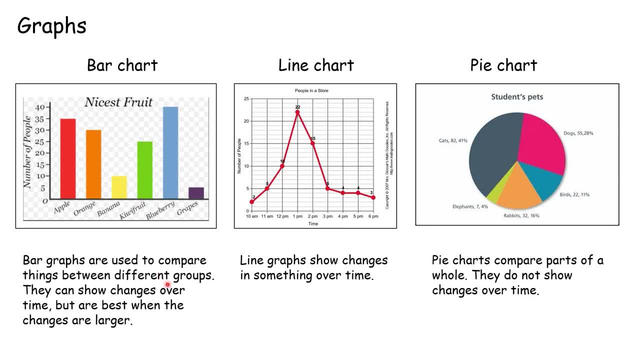 People liking different fruits. They can show changes over time, But best when the changes are larger. Line graphs show changes in something over time. It is continuous data. Every single point on this line has to mean something, And so perfect. Finally, we have pie charts. 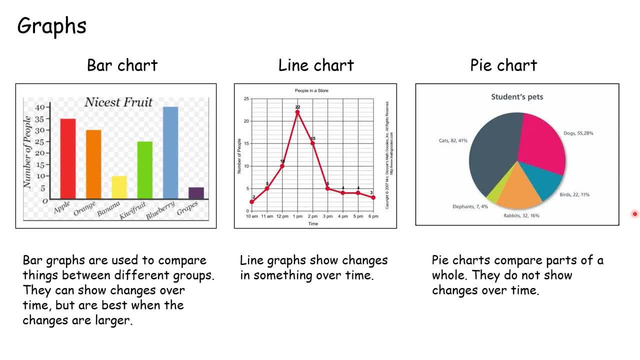 And pie charts compare different parts of a whole. They don't show changes over time. So here we have everybody's pets And then we're breaking it down into sections of people that have certain pets. So a little summary for charts and graphs. 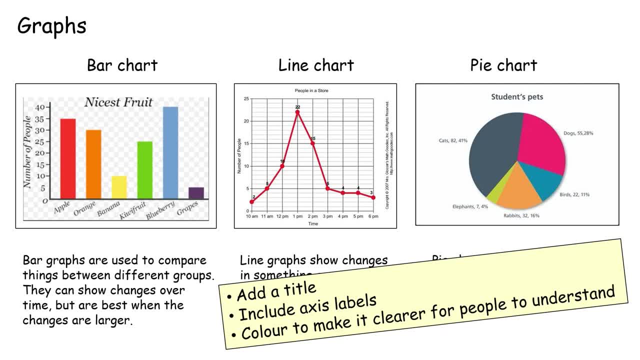 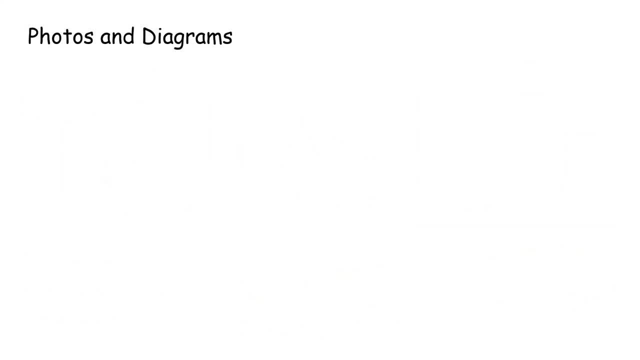 Make sure they've got a title, Make sure you've included your axis labels And include colour to make it clearer for people to understand. Finally, we've got photos and diagrams. Don't just bung a photo in without Labelling it to show people what you're trying to tell them. 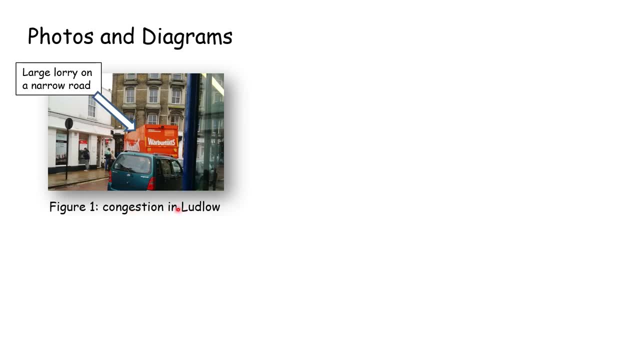 Titling it so that people can see what the photo is about And writing about the photo so that people can see its relevance. So figure one shows traffic congestion and lorries in Nudlow Town Centre. The lorries are causing vibration damage etc. etc. 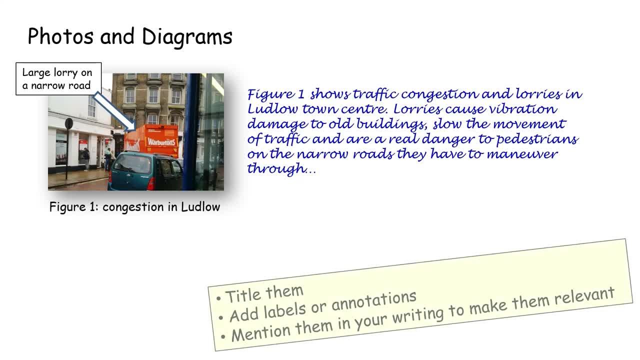 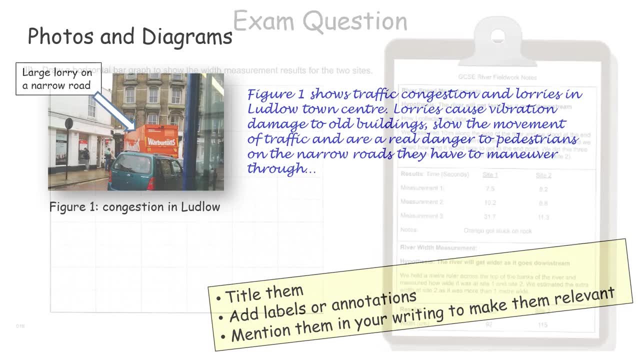 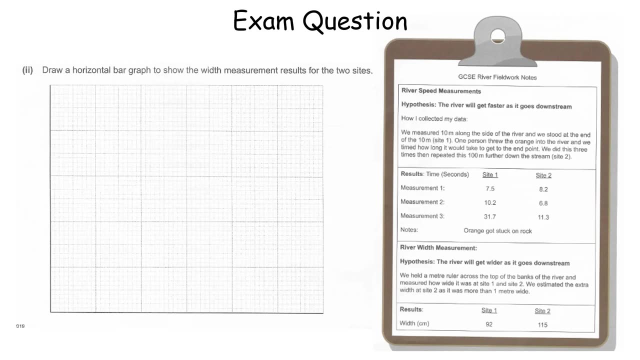 We've made that photo or diagram relevant Title. it Add labels and adaptations. Mention it in your writing. Now let's have a look at some exam questions to do with presentation. Here the candidate has to draw a horizontal bar graph to show the width measurement results for the two sites. 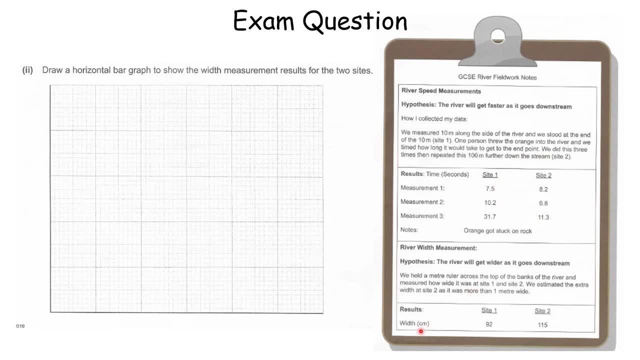 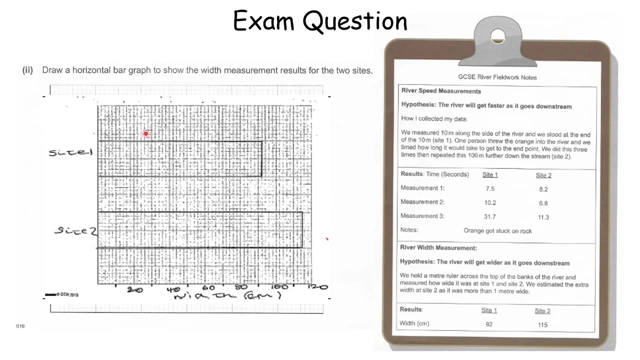 So go through the resource, Find width results, And you've got to do site 192, site 215 centimetres. Notice it says a horizontal bar graph. So what we do is we just turn our bars sideways. There is site 1 going exactly up to 92.. 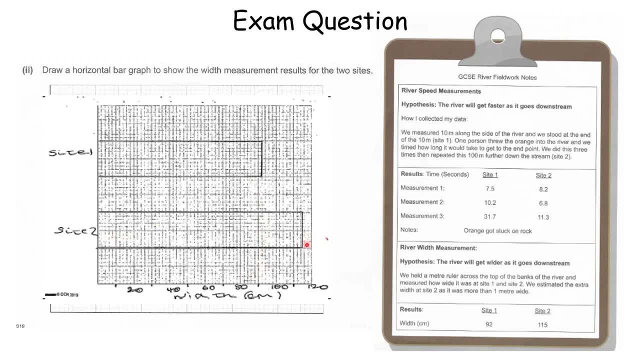 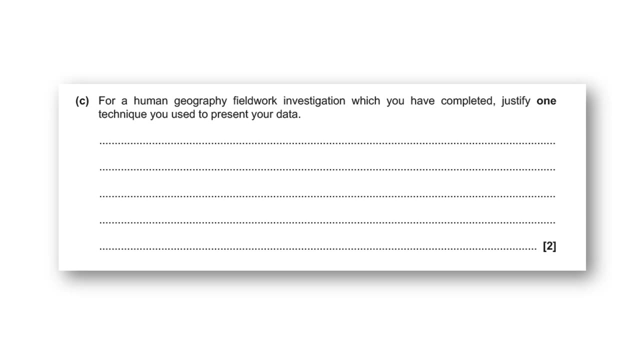 Here is site 2, going exactly up to 115.. You've written your units, You've labelled your axis full marks. Here's another one for human geography fieldwork, investigation: Justify one technique of data presentation. So you'd have to pick your pie chart or bar chart or whatever you've done, and say why it's suitable. 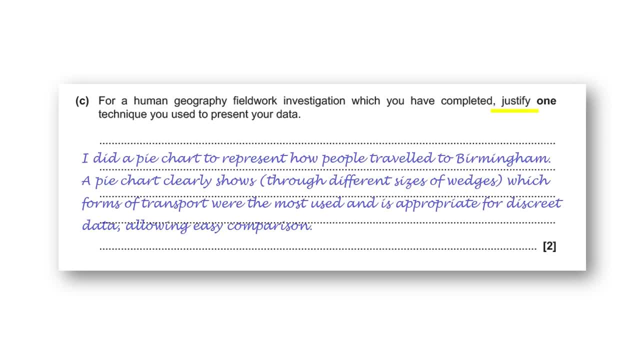 Justify is saying why So I did a pie chart. The pie chart clearly shows, through different sizes of wedges, which forms of transport were the most used, And it's appropriate for discrete data allowing easy comparison. So we focus there on how the pie chart is suitable to show the information. 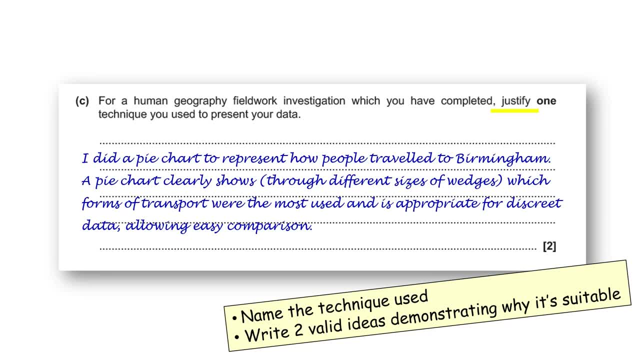 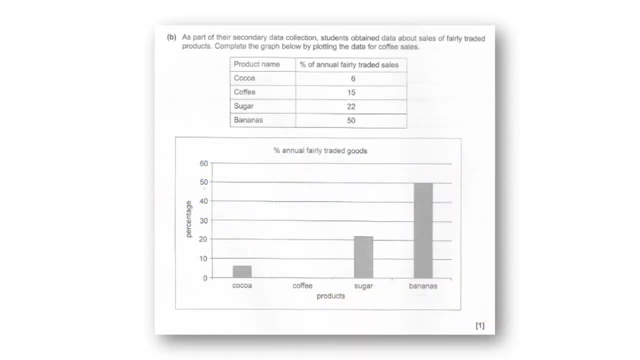 Name the technique. Write two valid ideas demonstrating why it's suitable Full marks. Here's another question. As part of the secondary data collection, students obtain data about sales of fairly traded products. Complete the graph below by plotting the data for coffee sales. 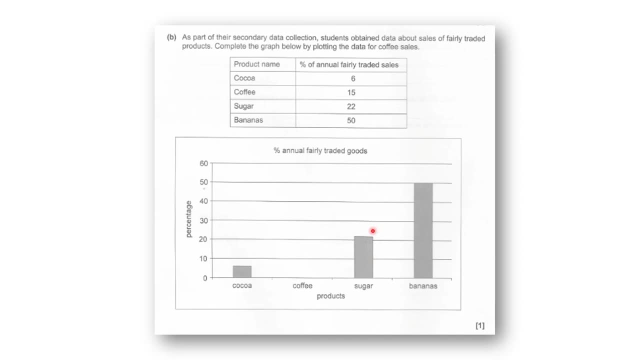 So we can see they've done a bar chart for bananas, A bar chart for sugar, A bar chart for cocoa. We've just got to put in the coffee 15.. So there it is. The ruling is: bar must be of similar width to the existing bars. 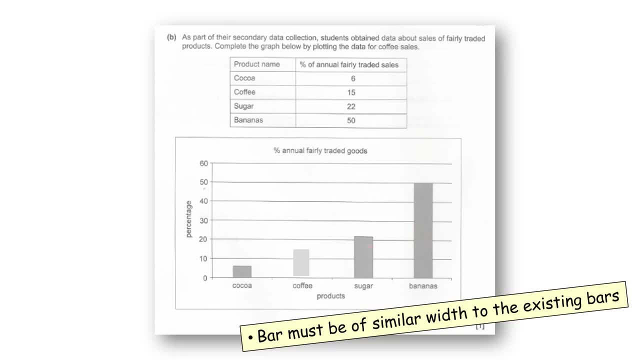 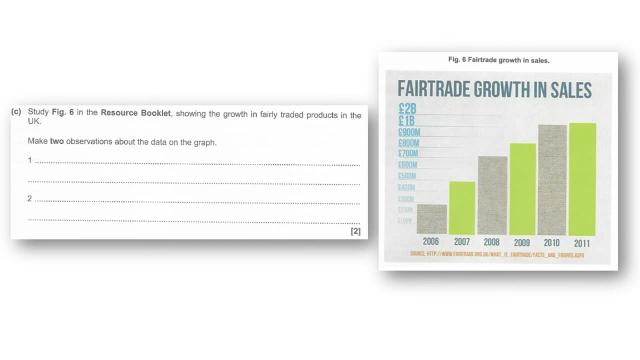 I'd also try and shade it a similar colour. Next question: Make two observations about the data on the graph. Now here is our graph showing fair trade growth In sales. you can see the bars are getting larger. So here are two observations. 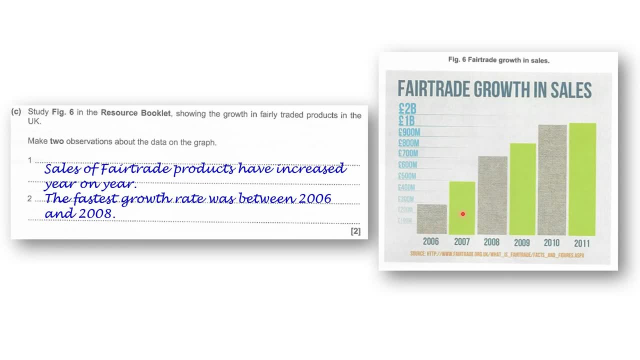 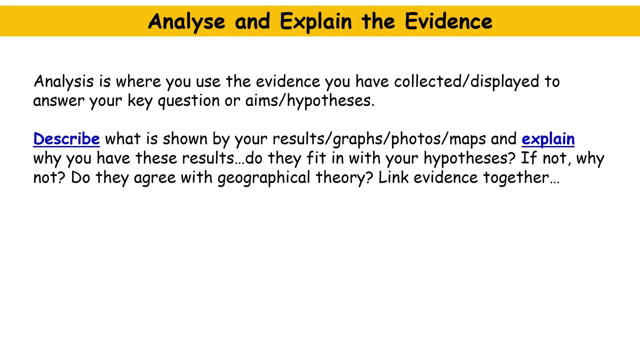 Sales of fair trade products have increased over the years. Yes, The fastest growth rate was between 2006 and 2008.. Yes, So the analysis section Analysis is where you use the evidence you've collected to answer your key question or aims or hypotheses. 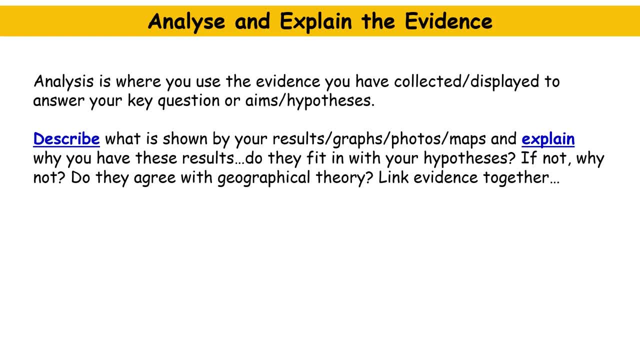 Generally we describe what is shown by the results- graphs, photos, maps we've got- And then you try and say why you've got these results. Do they fit in with the hypotheses? If not, why not? Do they agree with geographical theory? 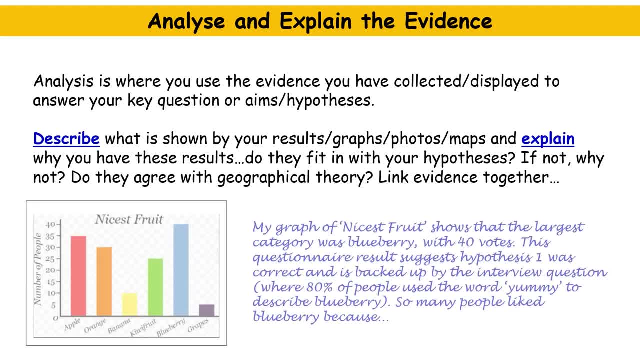 And you link evidence together. So here's an example. Here's our graph of nicest fruit. Let's see what we've done here. My graph of nicest fruit shows that the largest category was blueberry, with 40 votes. Now, that's just description. 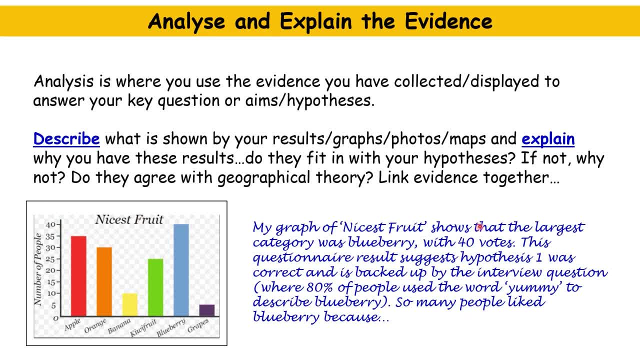 But I've used precise numbers, which is great. This questionnaire results: just hypothesis one was correct, So I've linked my graph to the hypothesis to show its relevance. It's backed up by the interview question, where 80% of people use the word yummy to describe blueberry. 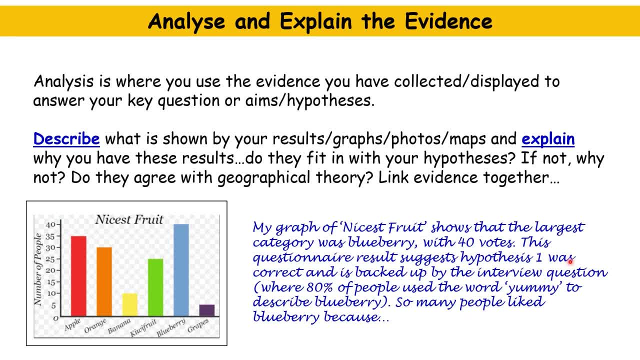 So many people like blueberry because. So I've done another two things here. To start with, I've linked this graph to an interview question And then I'm starting to explain here. So many people liked blueberry because, as well. So I've described. 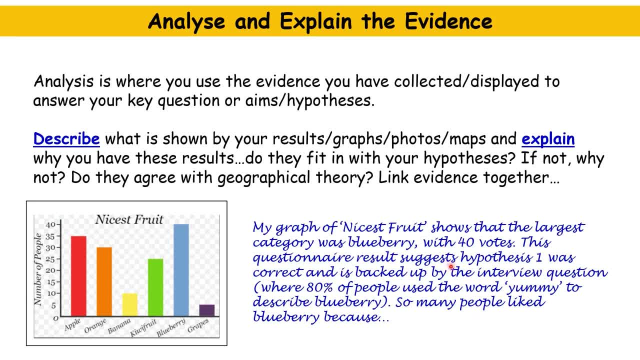 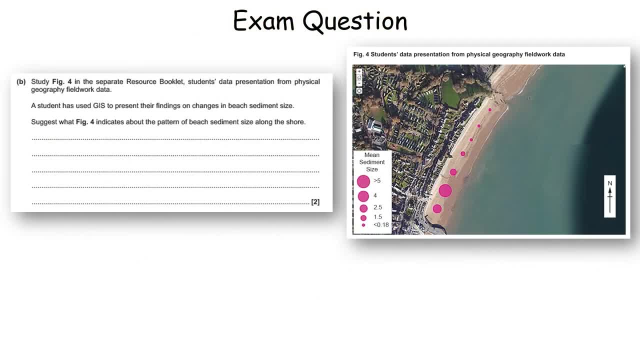 I've been precise, I've explained And I've managed to link my data together. Here's an exam question. So what does it say? A student has used GIS to present their findings on changes in beach sediment size. Suggest what figure four indicates about the pattern of beach sediment size. 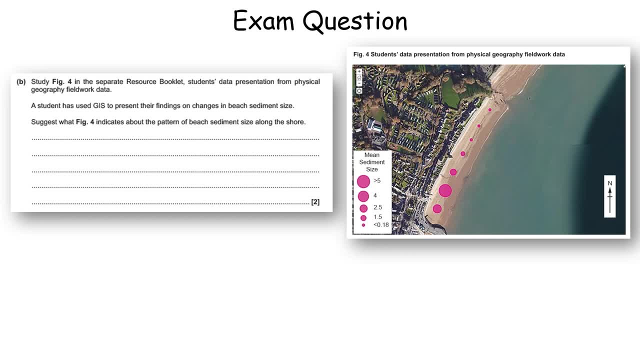 Along the shore. Now, when you see a diagram like this, just go to the key. So it says: mean sediment size. So the largest sediment size is the largest circle, The smallest is the smallest circle. So all we've got to do is just suggest two things. 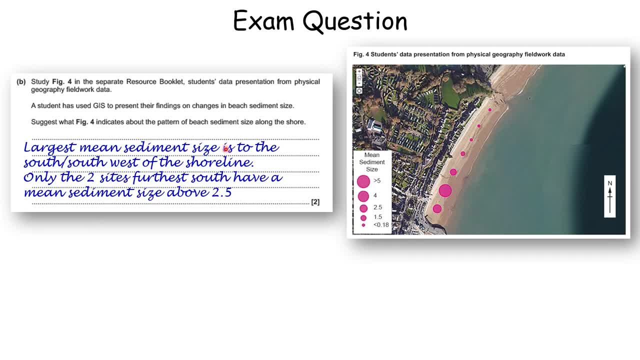 So largest mean sediment size is to the south or southwest of the shoreline. Yeah, true, And here's the smaller stuff. Only the two sites further south have mean sediment size above 2.5.. Again, true, Here's the largest sediment size. 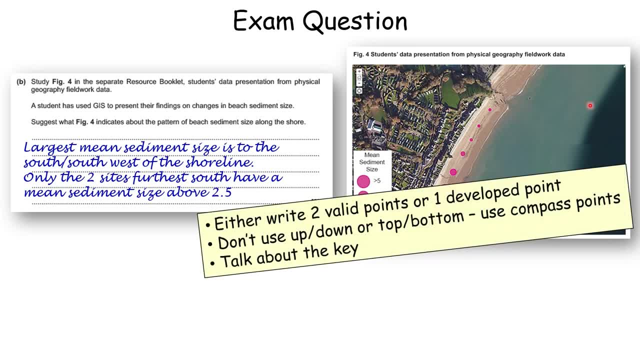 Now the rules here are: write two valid points or one developed. Don't use up, down or top bottom. Always use compass directions- north, east, south or west- And talk about the key in your answer. Here's another question. 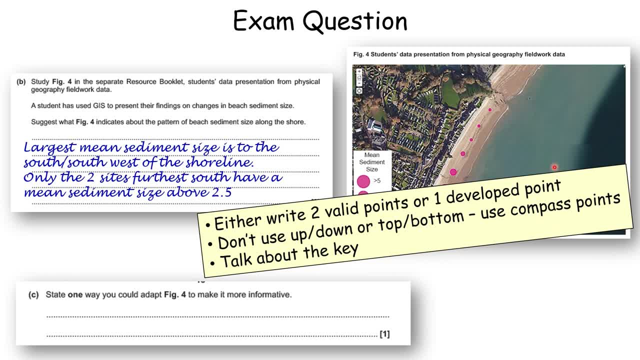 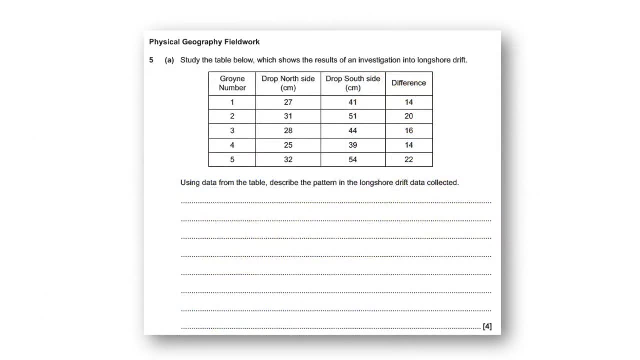 State one way you could improve this diagram to make it more informative. Well, you could insert a scale, You could add a title, You could add a location or show the direction of longshore drift, Just anything to improve it. Here's another exam question. 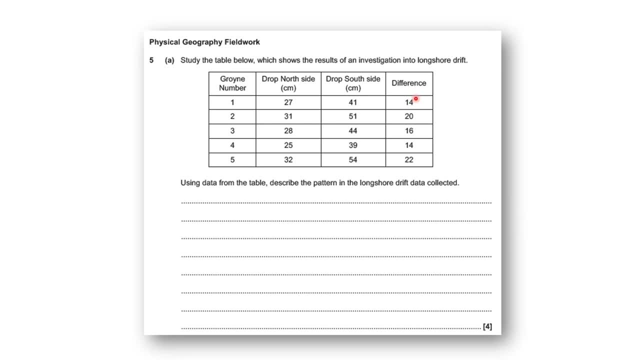 Using data from this table, describe the pattern in the longshore drift data collected. Now, because it says: using data from the table, mention these numbers, Describe pattern. What can you see within it? What can you see in the data? Oh, there's a greater drop on the south side than the north side. 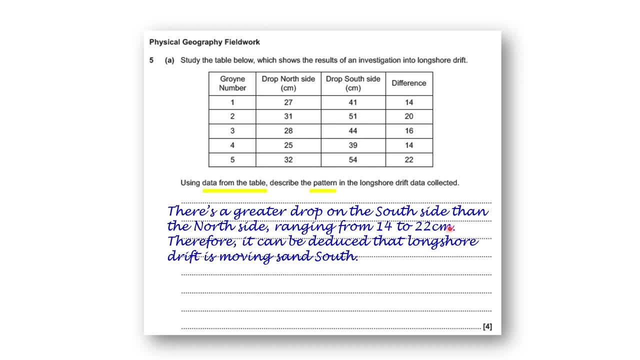 All these numbers are higher than these numbers ranging from 14 to 22 centimeters. Yes, Therefore, it can be deduced that longshore drift is moving sand south. Good, And that would be a very well-developed points. So what do you do? 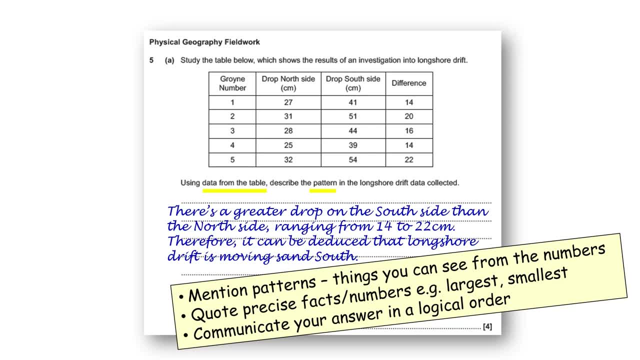 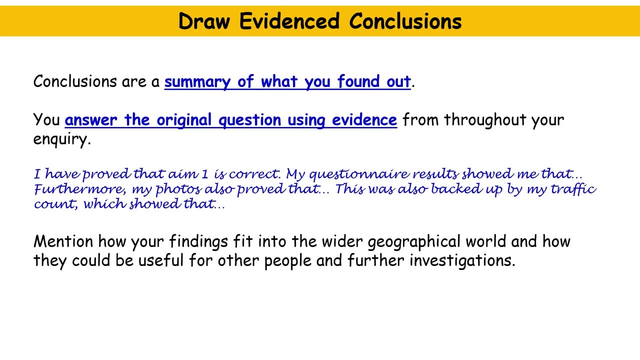 Mention patterns, things you can see from the numbers. Quote precise facts or numbers. You might say what the largest or smallest is. Communicate your answer in a logical order To get full marks. Drawing evidence to conclusions. A conclusion is a summary of what you found out. 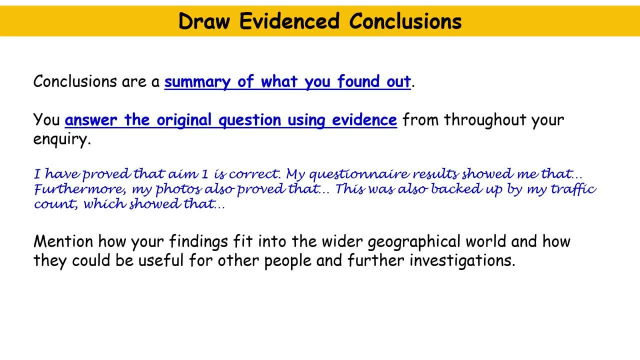 You answer the original question using evidence from throughout your inquiry. So the sort of thing you might write is: I've proved that aim one is correct. My questionnaire results showed me that. Furthermore, my photos also prove that. This was also backed up by my traffic count, which showed that. 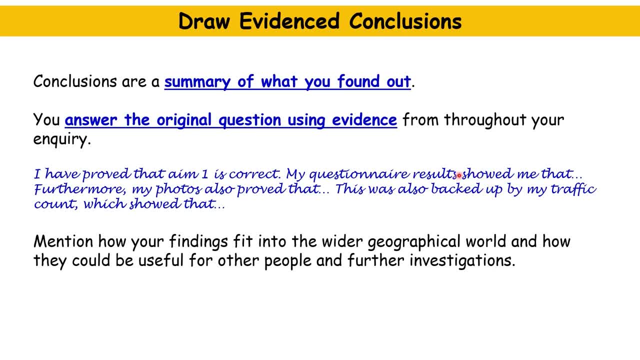 So we're drawing on evidence from throughout Project in order to answer our original aim or question or hypotheses. Then you'd mentioned how your findings fit into the wider geographical world and how they could be useful for other people and further investigations. Here is a past exam question. 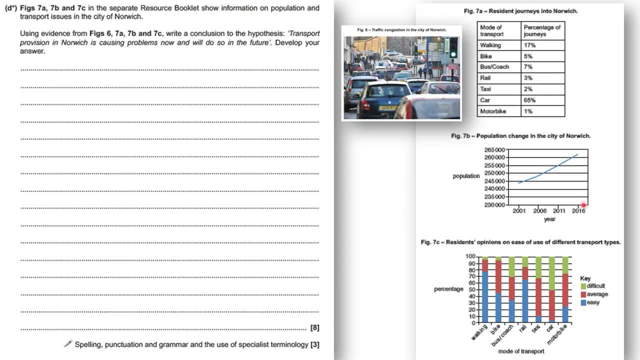 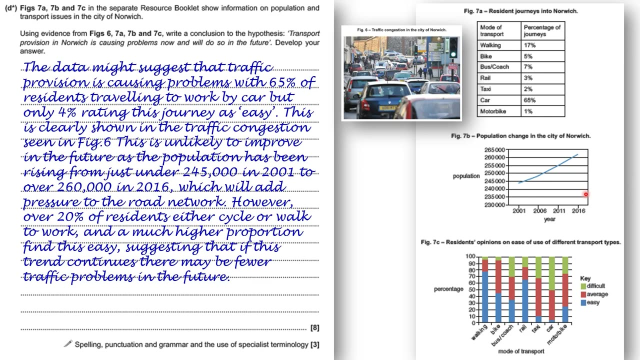 You're provided with these resources, and then it says: write a conclusion to this hypothesis. Here is a very- Here is a very well developed answer. If you want to pause the video, you can in order to read it, But what they've put in there is precise figures. 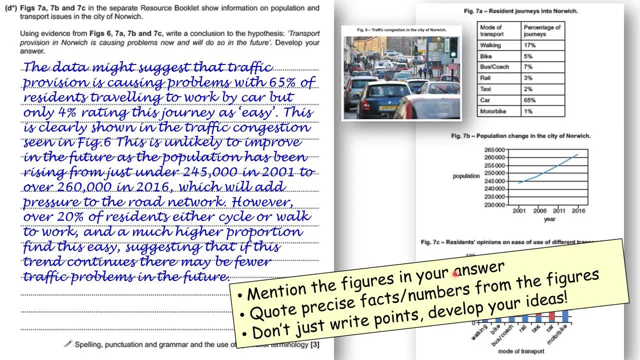 They've. they've put precise facts and numbers from these diagrams. You want to say figure 7A shows and pick some of these numbers Figure 7B shows and work out the population compared to the year on this graph, etc. They haven't just written points. 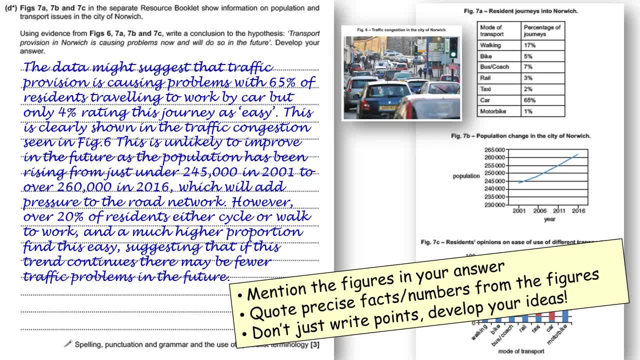 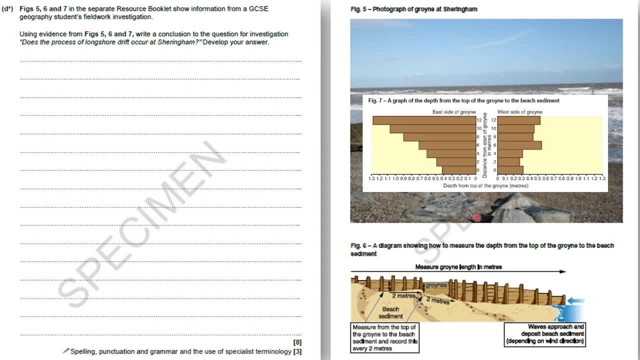 Again, the ideas are really well developed. Here's another exam question. Here are resources that were provided. Here's the exam question saying: write a conclusion to the question of investigation. Does the process of longshore drift occur at Sheringham? Develop your answer. 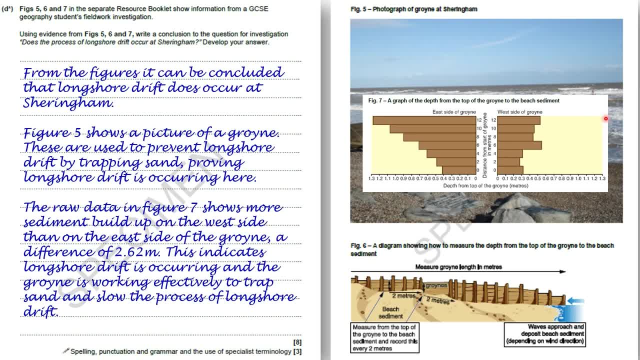 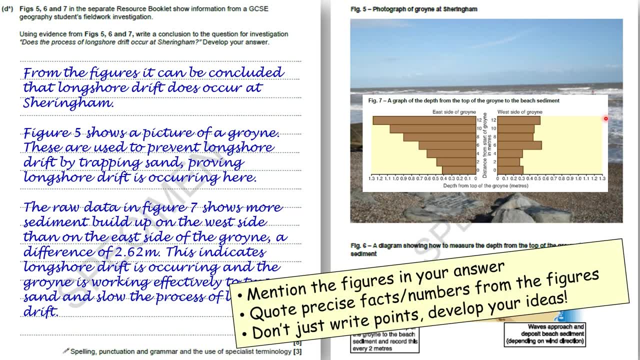 Again, here is a superb answer, Very, very well developed. Again, if you want to pause the video, If you want to pause the video and take a look through that. But what have they done? They've mentioned the precise figures. 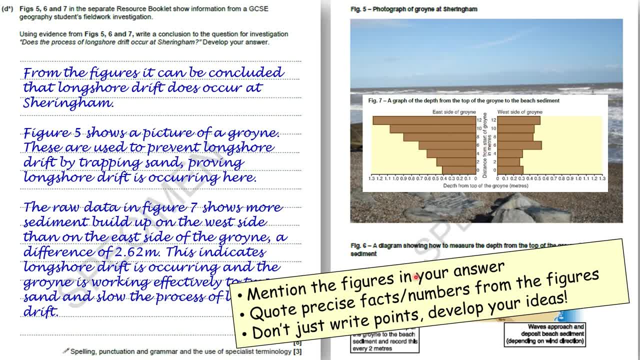 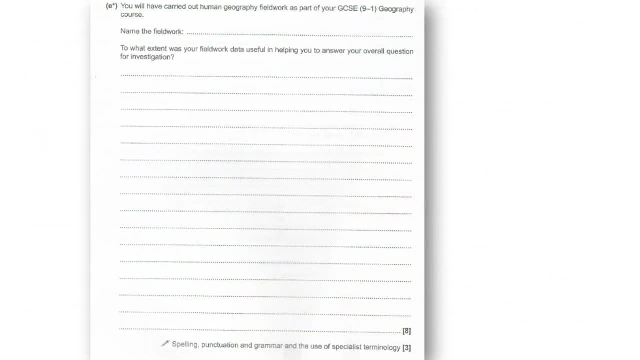 Figure 5 shows. figure 6 shows Again: they've quoted precise facts and numbers from these figures And then they haven't just written points. There's very, very well developed ideas in order to get full marks. Finally, another example. 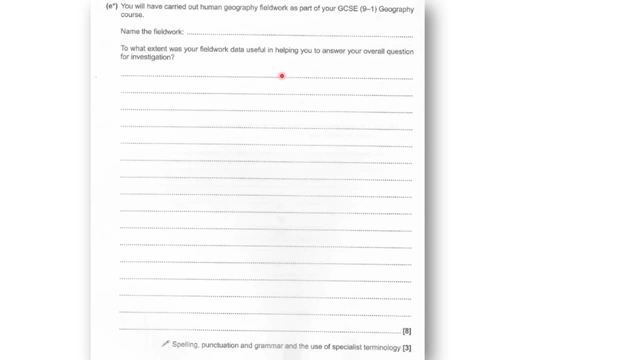 To what extent was your fieldwork data useful In helping you to answer your overall question for investigation? Now, most likely in the exam they'll be asking you about an example that they've come up with, like the previous ones. But again, let's imagine there's our fieldwork title. 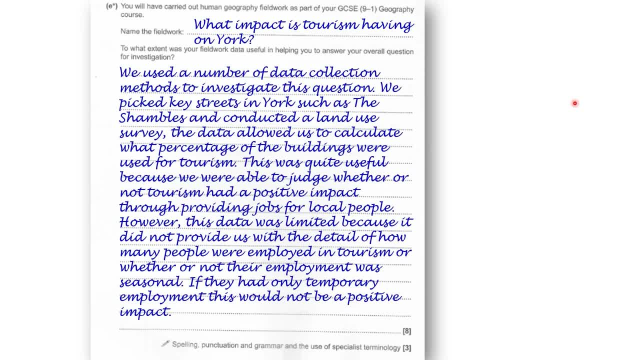 What impact is tourism having on York? There is a perfect answer that the examiners were really really happy with. Again, you can pause to have a look at this, But they stated what data they collected. They've mentioned and developed How it was useful to them in the project. 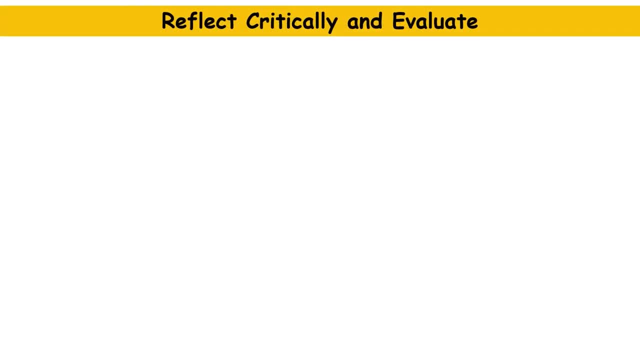 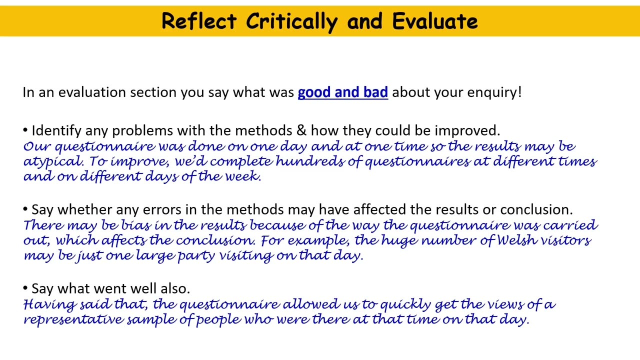 The final section of an inquiry is where you evaluate what went well and what you could improve. So you write what was good, what was bad about your inquiry, Identify any problems you had with the methods and how they could be improved. So, for example, our questionnaire was done on one day and at one time. 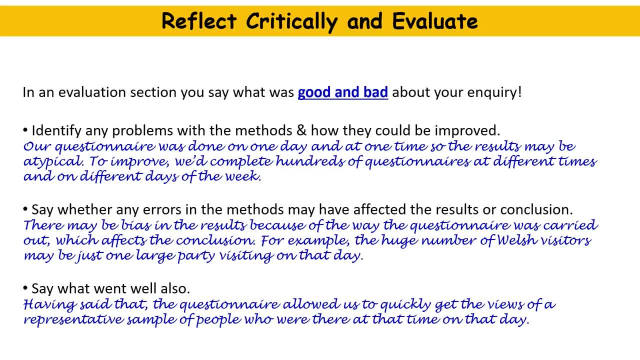 So the results may not be usual or normal. To improve, we'd complete hundreds of questionnaires at different times on different days of the week. Brilliant. Secondly say whether any errors in the methods may have affected the results or conclusion. There may be bias in the results because of the way the questionnaire was carried out, which affects the conclusion. 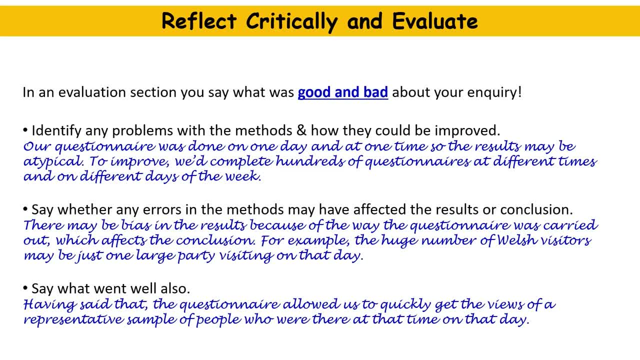 For example, the huge number of Welsh visitors- maybe just one large party- visiting on that day- Great. Finally, also say what went well. Having said that, the questionnaire allowed us to quickly get the views and represent a sample of people Who were there at that time, on that day. 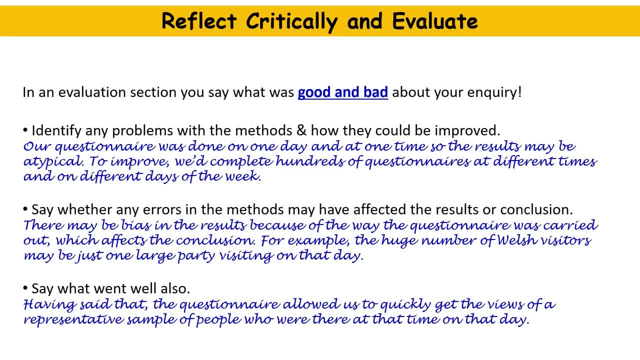 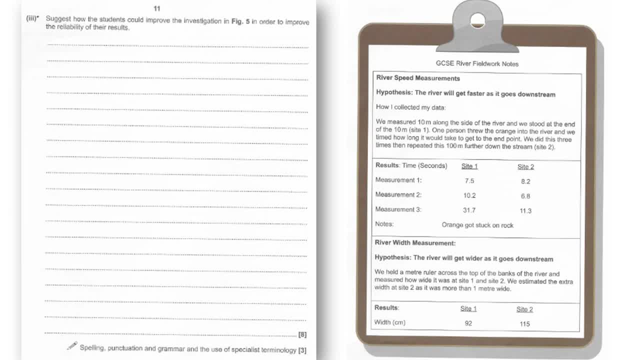 So, with your evaluation, say what was good, say what was bad. Here's an exam question. They've provided us with GCSE River Fieldwork notes here And it says just how students could improve the investigation in order to improve the reliability of their results. 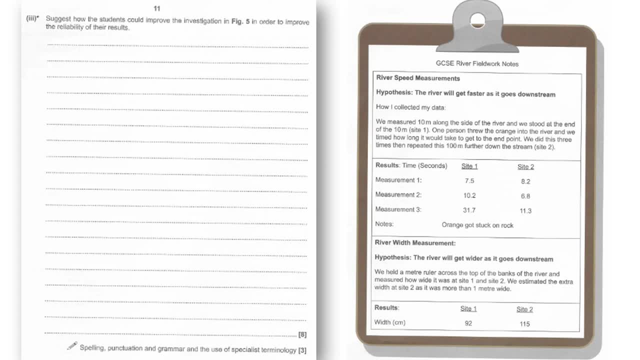 Now the thing with this is have a really good, slow, thorough read through it. Try to find any problems that you can see any ways to improve, And then that's how you would answer it. So just look here. We held the meter ruler across the top of the banks of the river, measured how wide it was at site one and site two. 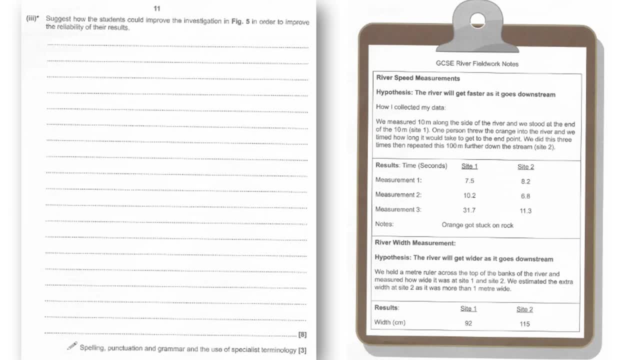 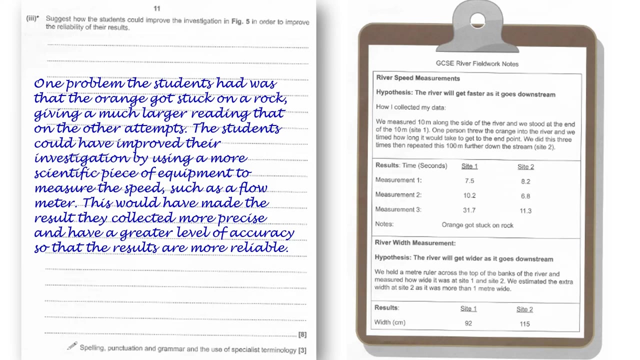 We estimated the extra width at site two as it was more than one meter wide. So right this side, they were just guessing the width, which means it's less reliable and less accurate. Here's a good answer. One problem students has was that the orange got stuck on a rock, giving a much larger reading than on the other attempts.